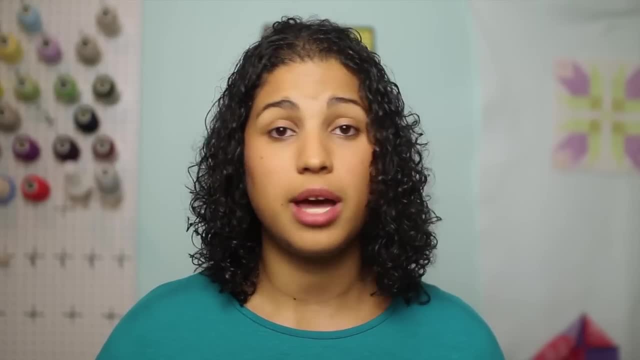 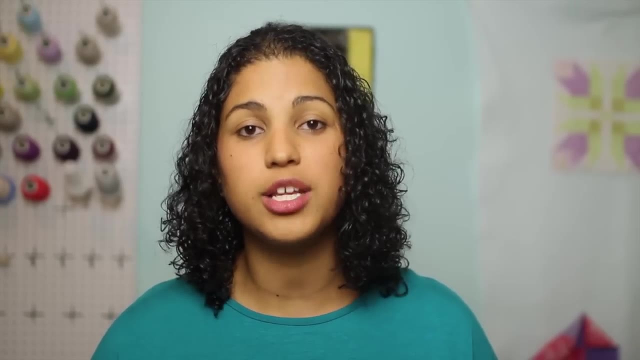 me follow what she's doing, So I can do it correctly as well and I can learn how to use the things okay. So, as a parent, feel free to make that decision on your own, whether you choose the same route or you just want to use more child safe or child appropriate items. So let me start off. 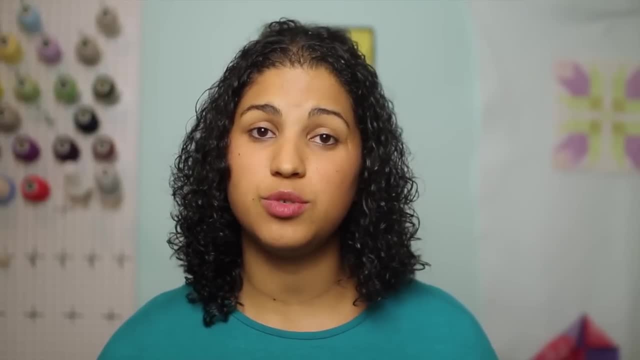 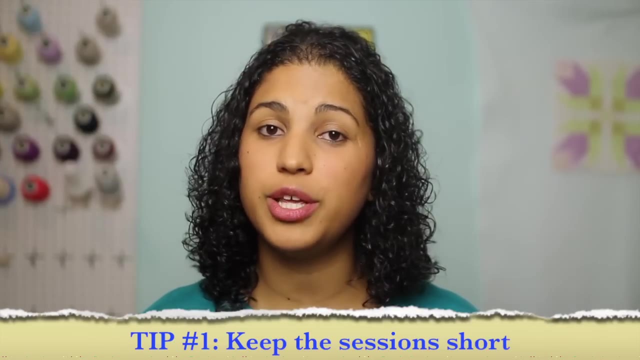 by giving you three quick tips of things I like to incorporate in my sewing sessions when I'm teaching my son. The first one is to keep the sessions short. Young children don't have that long of an attention span and my son's only three, so I definitely don't. 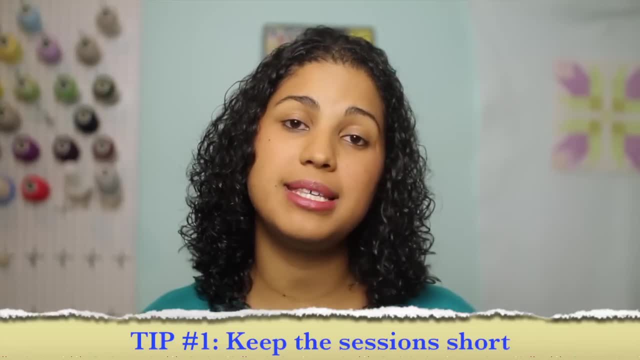 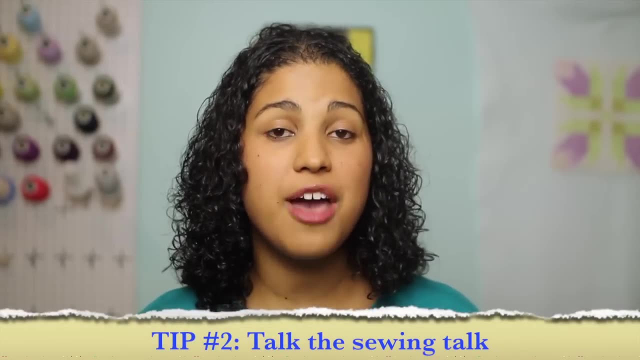 want to burn him out or get him too bored with the machine, so I keep my sessions with him to no longer than five, maybe ten minutes. Now. the second tip is to speak the sewing terminology. Every step of the way, I'm pointing out something on the machine mentioning its name: presser, foot needle, sewing pins. 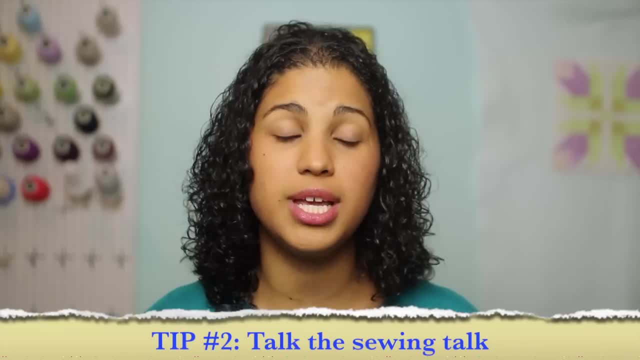 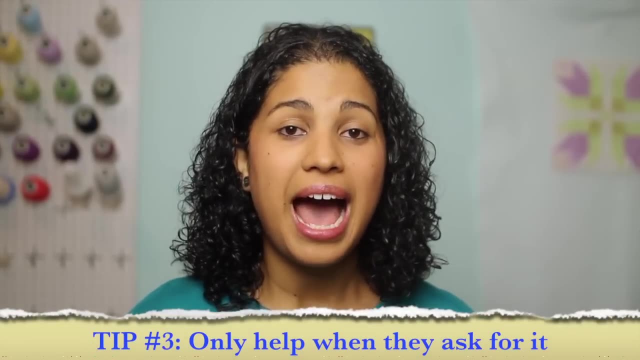 scissors, thread, you know. throw out the words there so they can pick it up and start learning everything there is to know about working on their own sewing projects. And the third tip is to let the child do what they can. With my son, I go through the first. 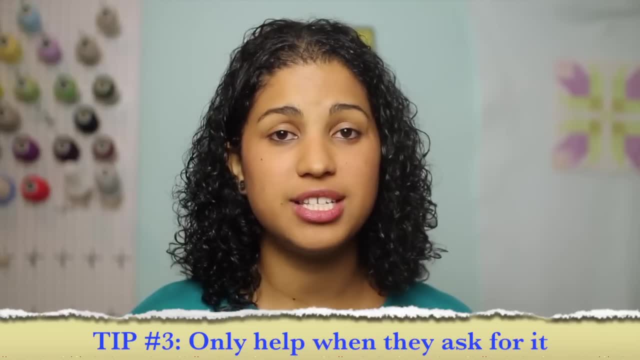 time I show him how everything works and where everything goes, and then after that I just let him do it himself. If he can't do it or he gets stuck, then he'll ask me for help and I'll just let him do what he wants to do, and then I'll just let him do. 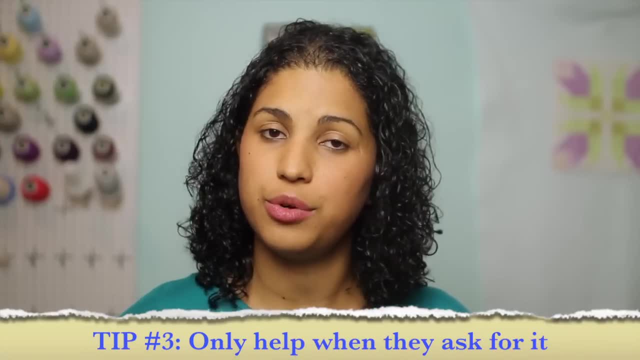 what he wants to do, and then I'll jump in and help him. Otherwise, I let him do simple tasks and things that I know he can do. So now I'll leave you with the video of me teaching my son how to use his sewing machine. 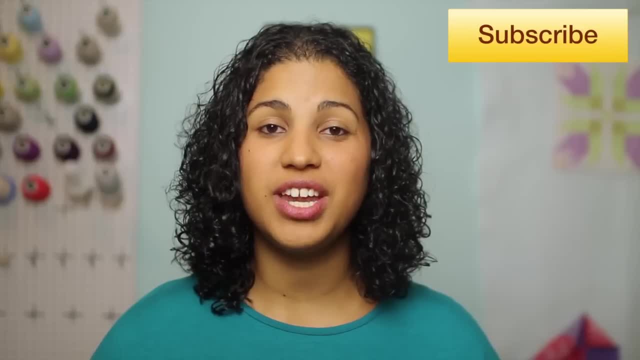 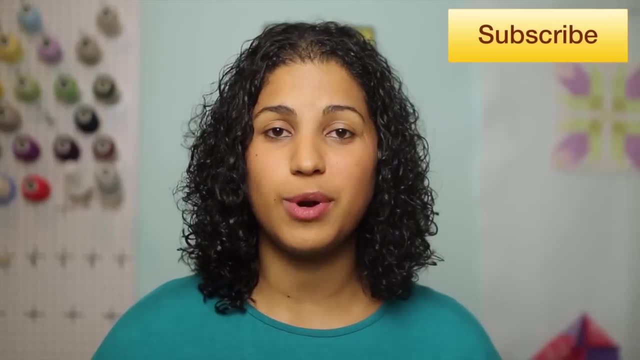 This is only his third sewing lesson and if you have any questions of anything you see in the video, feel free to drop me a question underneath this video here on YouTube. Take notes, get some ideas. I hope you get some inspiration from it and that you'll take. 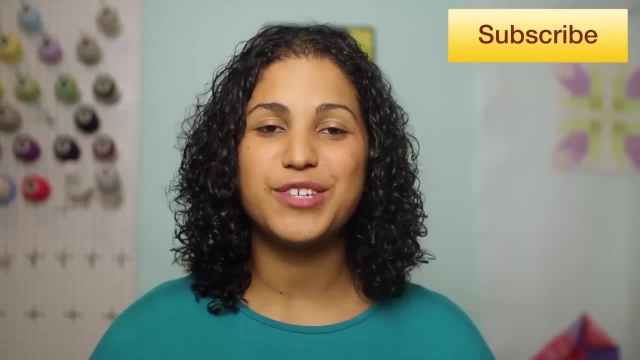 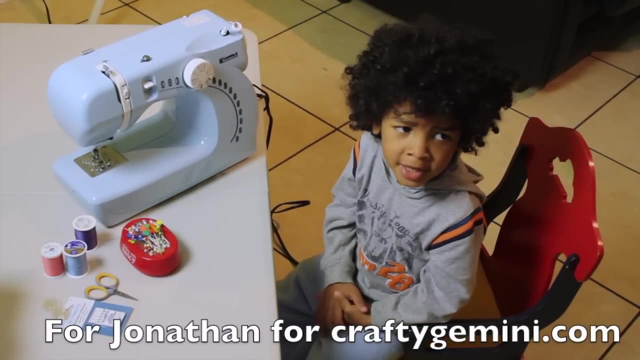 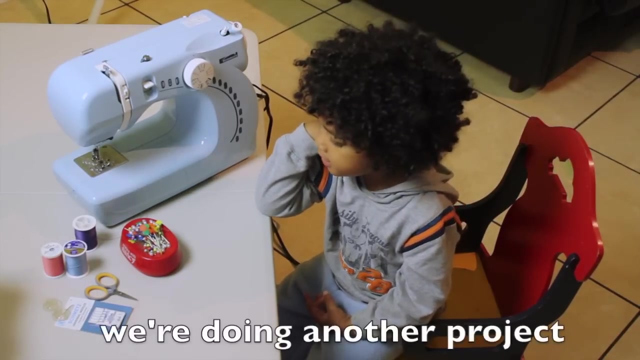 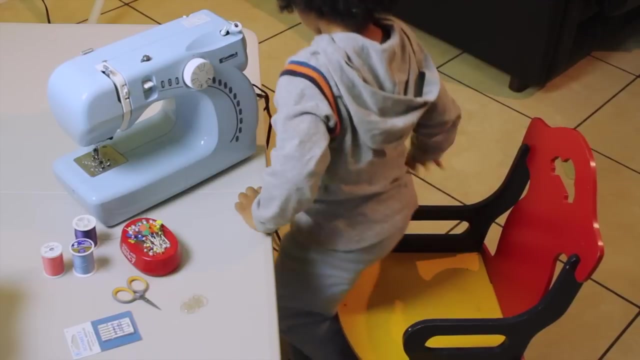 the step to teach a child in your life how to use a sewing machine. Thanks for watching and I hope you enjoy the video. Bye. So can you tell your camera friends, what do you need to start sewing with your first sewing project? What do you need first? What is that big machine there? 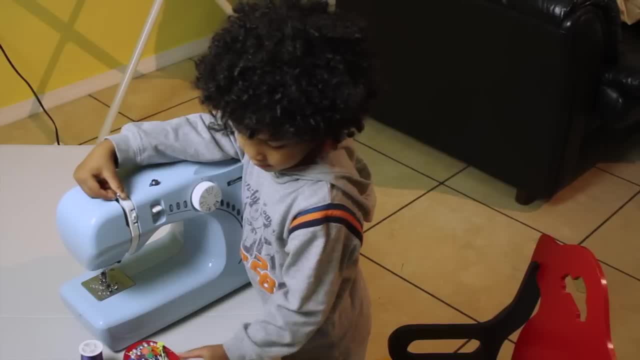 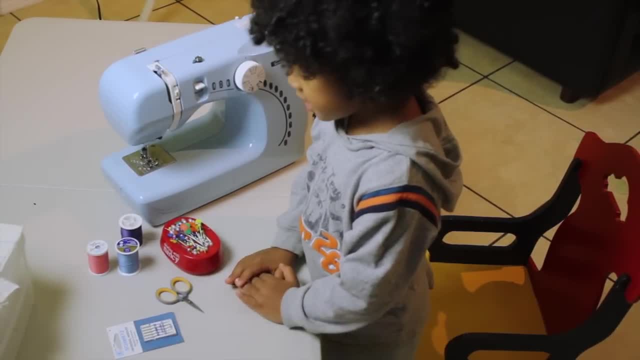 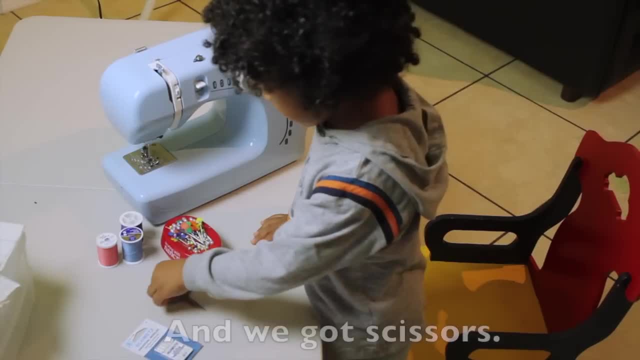 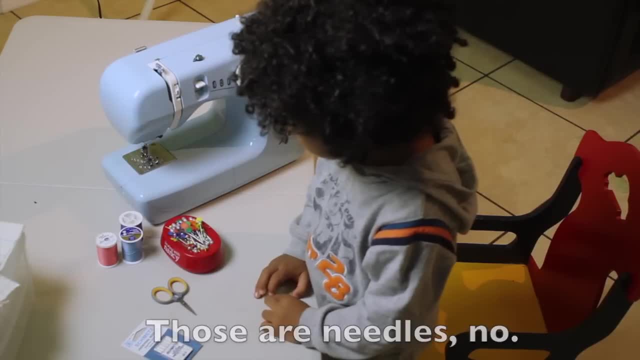 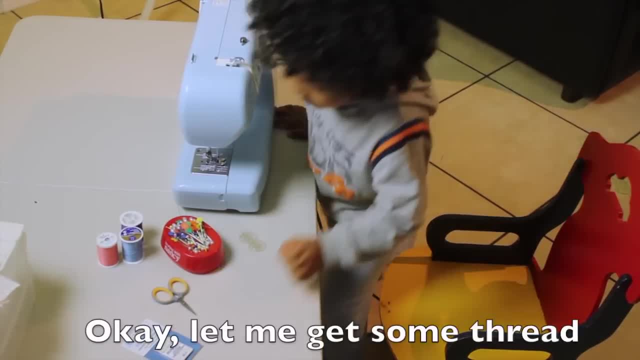 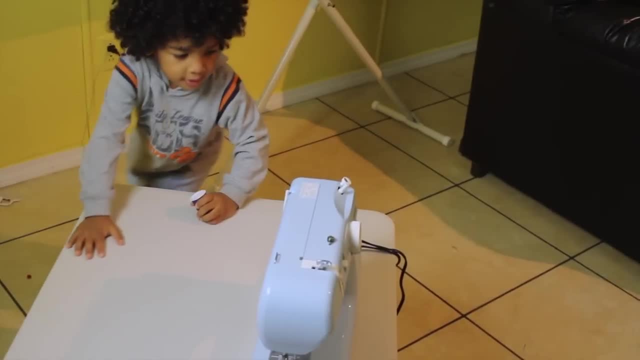 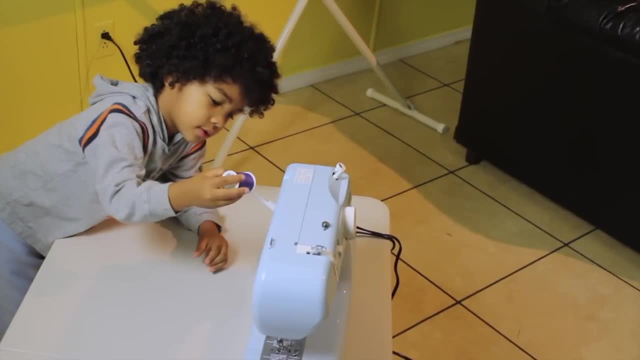 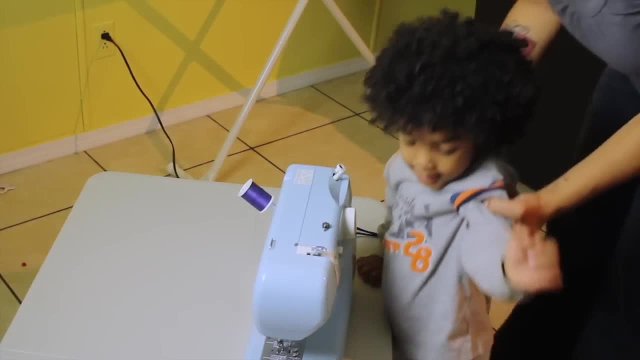 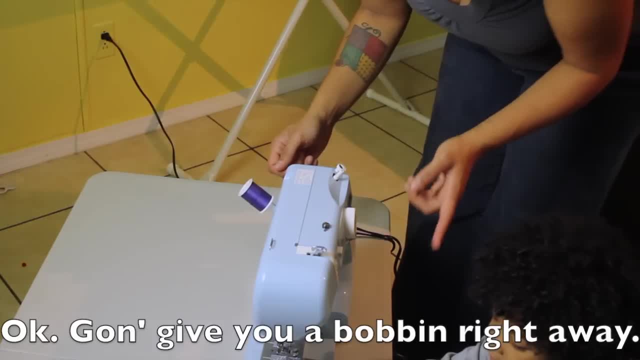 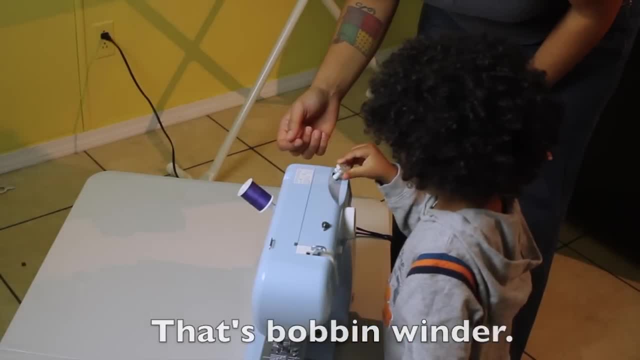 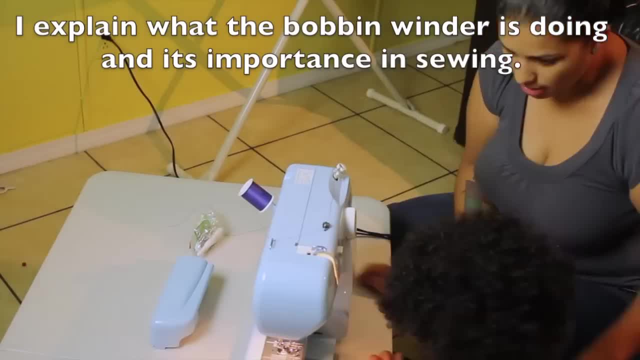 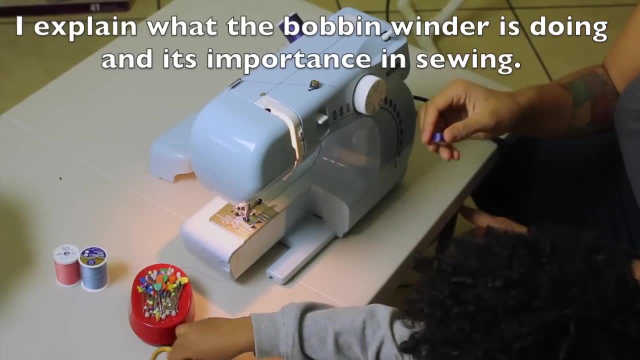 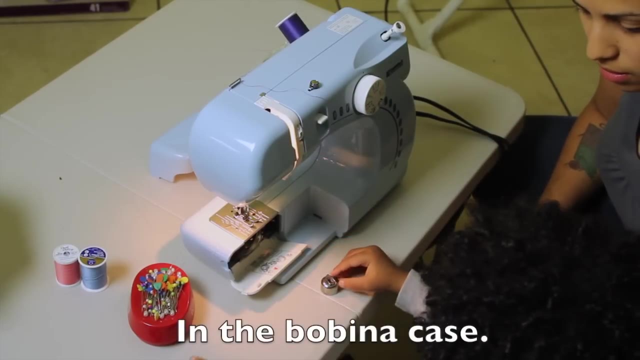 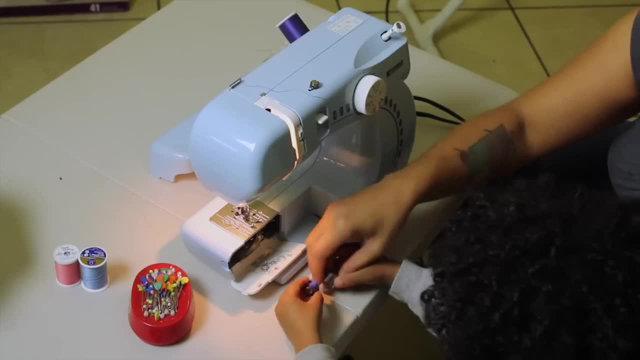 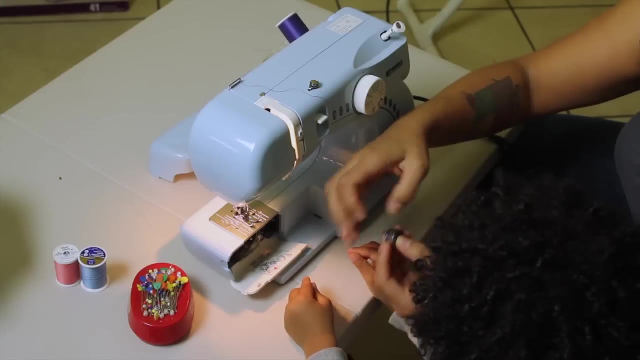 So let's get your new bobbin, the purple one, right And put it in there. Good job. Now I'm going to show you here. This thread needs to go through here. You're going to put it right through there until we hear it snap. 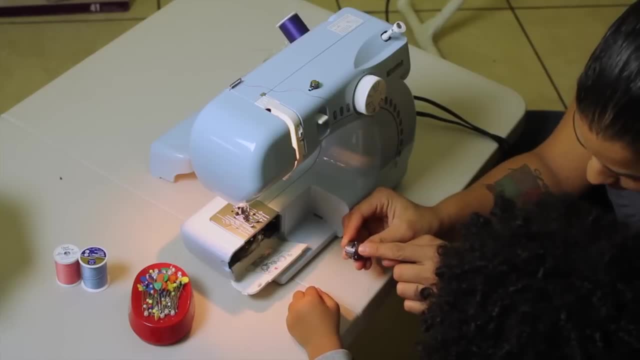 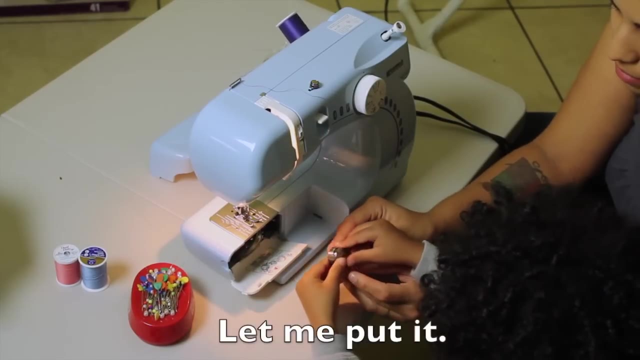 Like that. Okay, And remember I put this little handle has to match up where in there In the tiny tiny circle. Okay, Let me pick it Until we hear it snap right, Push it, Snap Like that. 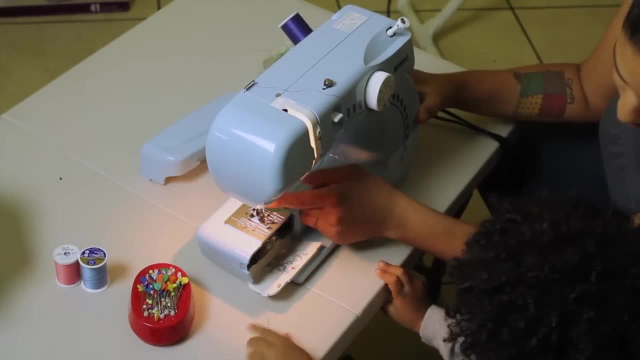 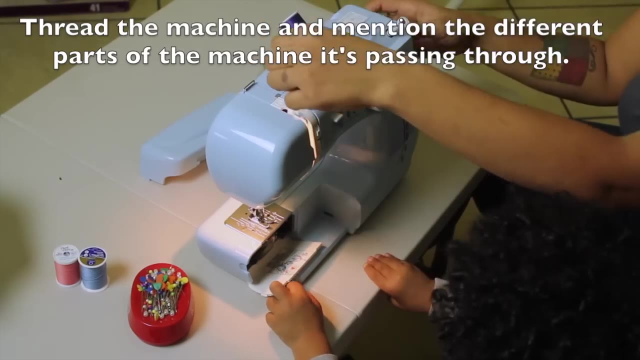 There you go. Okay, Now we have a thread coming down here. Do we have thread in this needle yet? No, We got to put thread there too, Okay, So it's going to snap up here. Okay, It's going to snap. 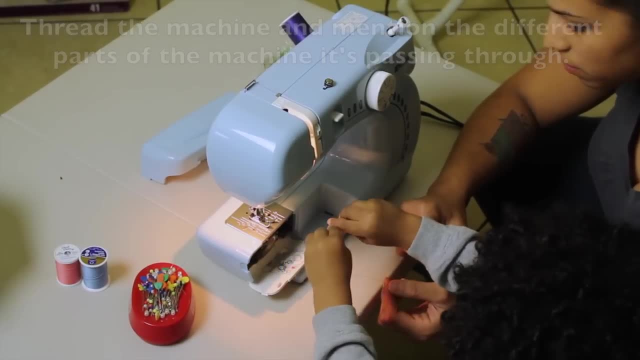 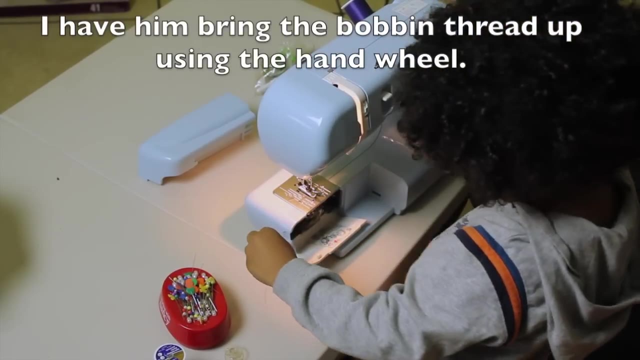 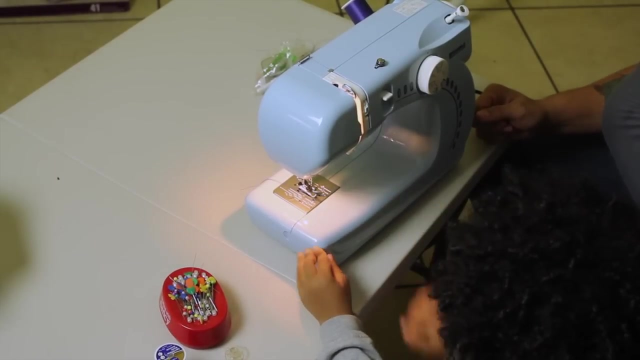 We're going to put thread in there And it needs to go through here too. Okay, So we're going to screw that in And we're going to close it up. Okay, Then we're going to put thread in there, Okay. 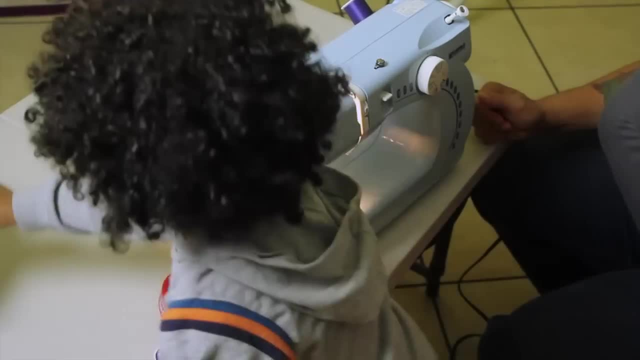 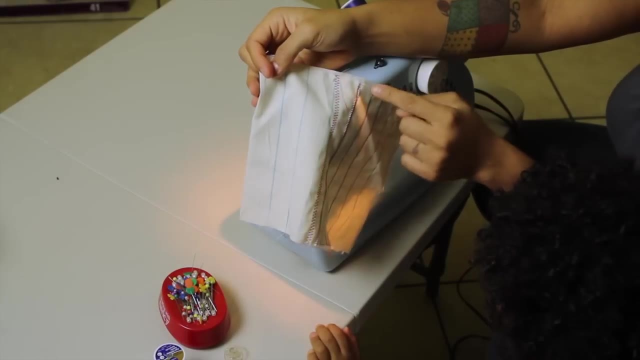 We're going to close it up And that's our bobbina. Okay, Close it up. Put on the front part. what I have here is just a piece of muslin, and I just took one of his markers and drew some straight lines on it, and then I have him try and follow. 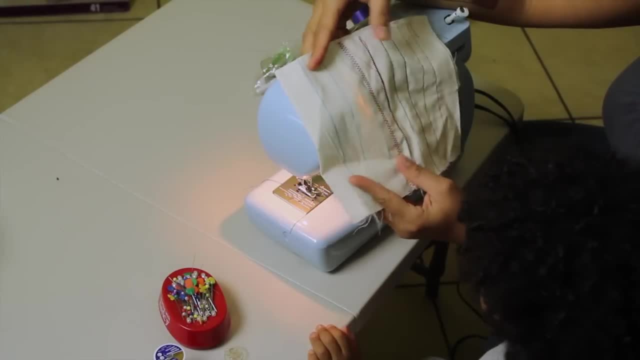 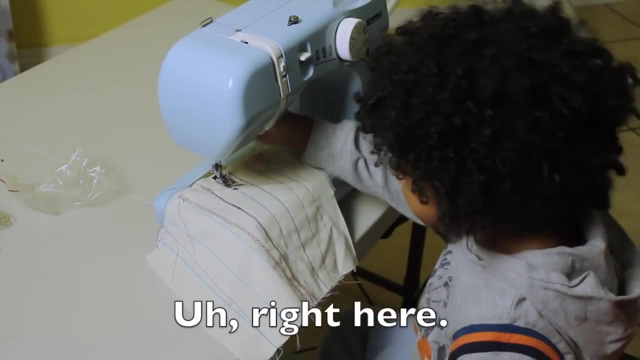 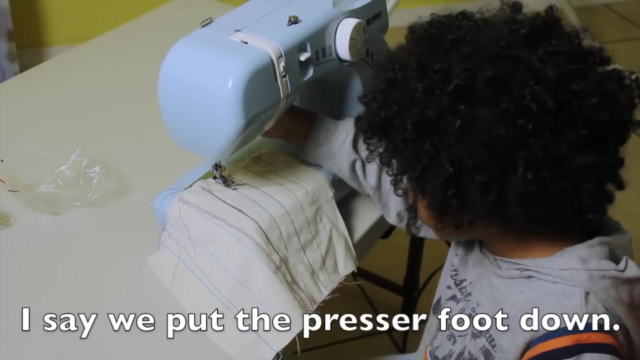 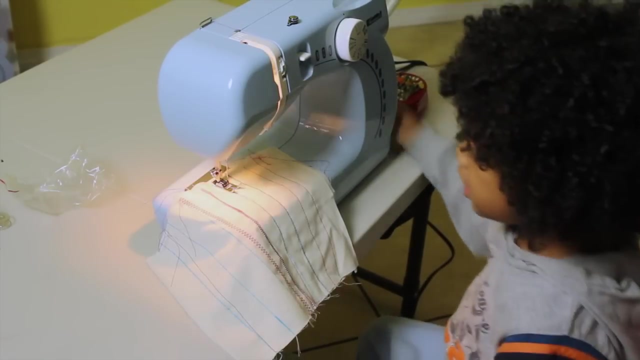 these lines stitching straight. they're not gonna be perfect at the beginning, of course, and just the more practice they get in, the better, I think. okay, so we're ready to start sewing. where are you gonna put your fabric? okay, what's the next step after we have our fabric in place? perfect, okay, go for it. and where? 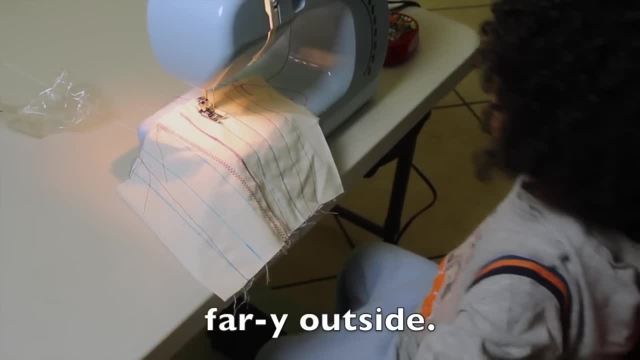 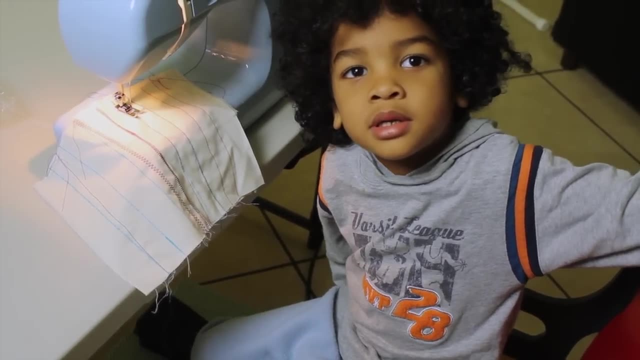 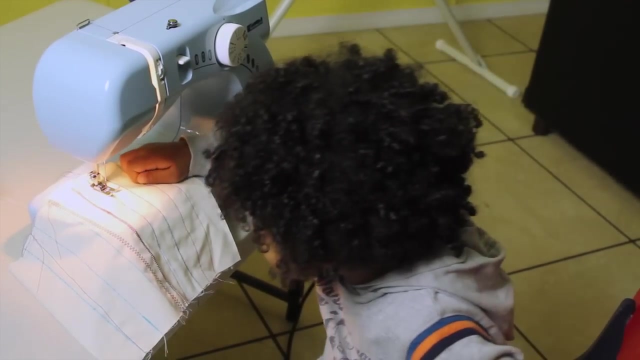 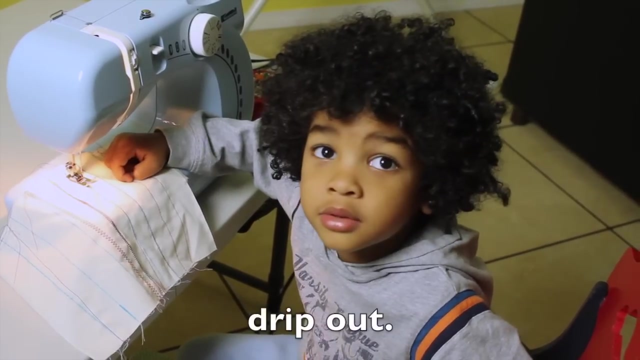 are you putting your fingers at, just like outside, far away, you're keeping your fingers far away from the fabric and then you're going to start sewing. from what part of the sewing machine? yeah, because what can happen if that needle gets your finger okay and blood gonna drip out. okay, you're right, that's.